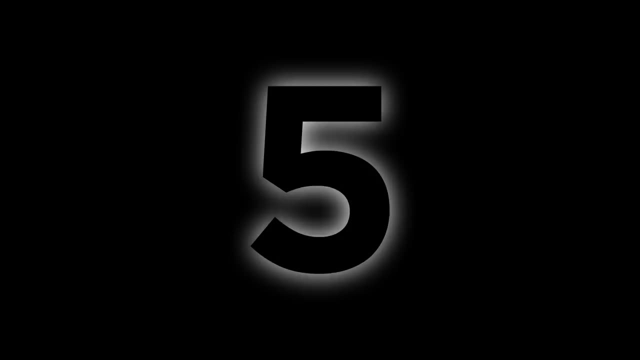 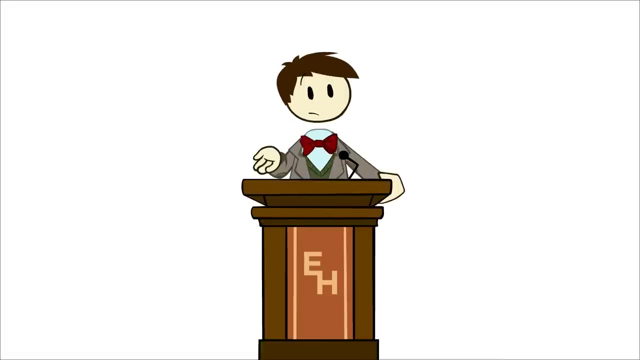 What if Euclid wasn't right? For centuries, people had beaten their heads against the problem of trying to prove postulate 5.. But what if? Instead of doing that, what would happen if we just accepted that postulate 5 couldn't be proven? It wouldn't make Euclid wrong, but it would mean that Euclid wouldn't be true. It would mean that the Euclidean view of the world, upon which we had built so much, wouldn't be the only view. What madness would we unleash if we peered at the world through some other lens? 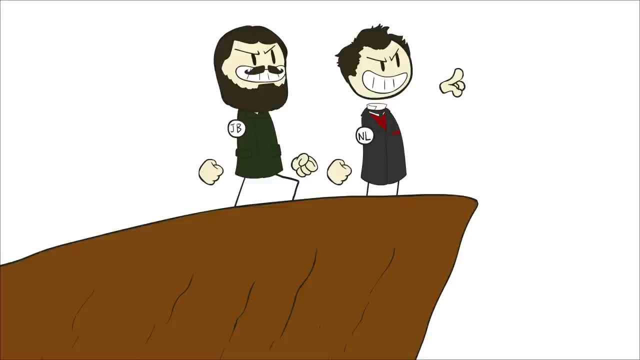 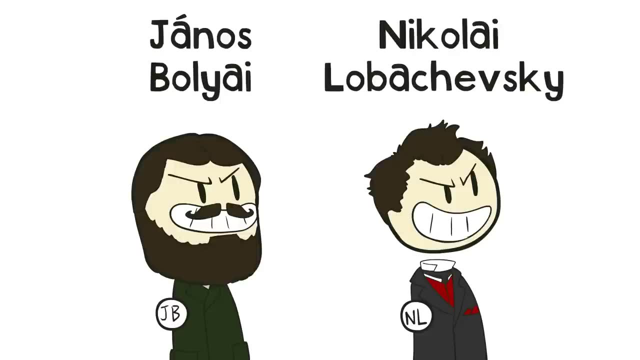 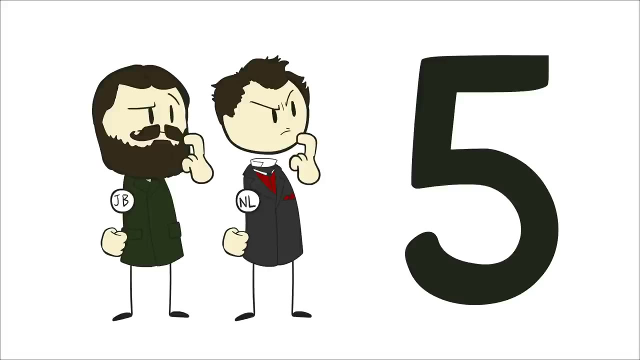 Well, two figures at least were willing to sin boldly and peer past where all other human reason had taken us. Their names were Janos Bolyai and Nikolai Ivanovich Lobachevsky. The differences in their work is a bit esoteric, but at its heart both of them delved into alternate possibilities for postulate 5.. 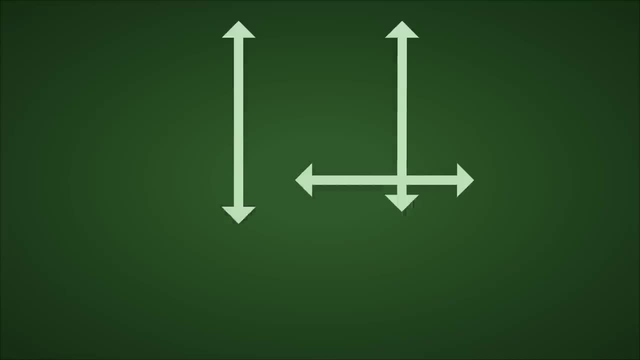 You remember how, in Euclid, we basically said that if you put two lines across another line and their interior angles add up to 180 degrees, the two lines would never get any closer or further away from each other, thus giving us our traditional definition of parallel lines. 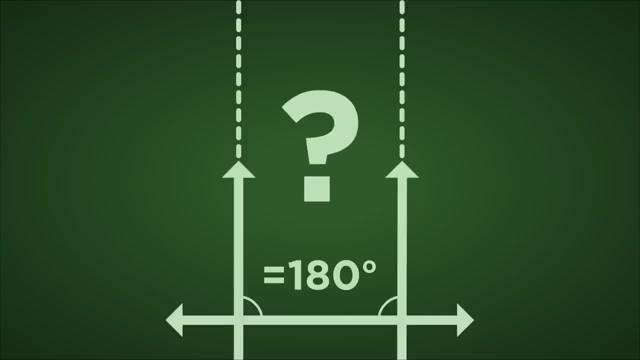 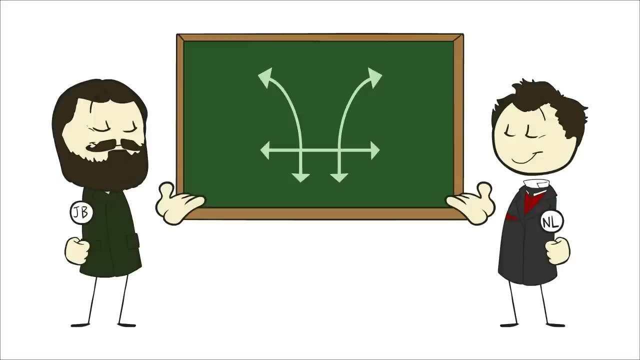 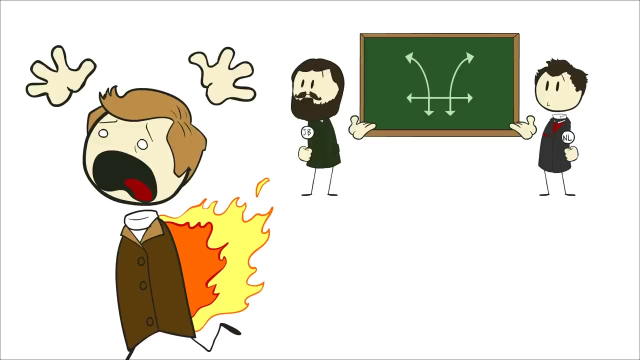 Well, what other options are there? Those lines either do get closer to each other or do get farther away. Bolyai and Lobachevsky introduced the case where our parallels could curve away from each other, And with that one small change they unleashed a torrent of madness. 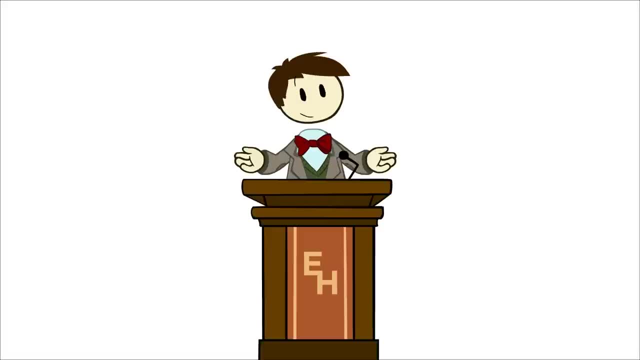 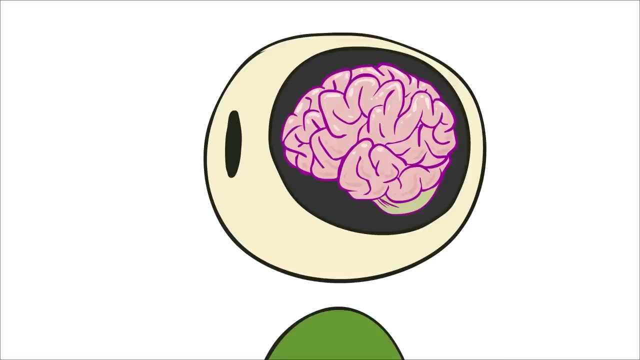 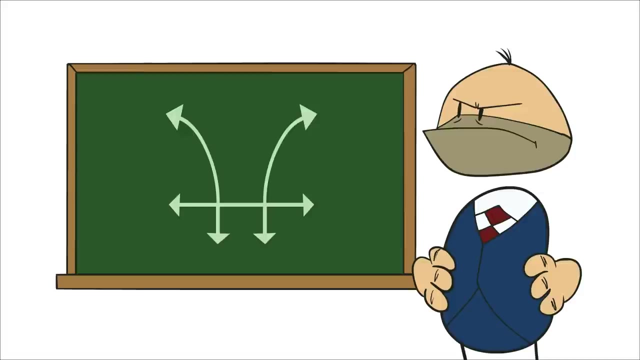 And it is all as logically valid as Euclid. It's all as internally consistent as Euclid, But to a mind that has been trained to understand the world through a Euclidean model it is a little bit brain-melting. The stuff that happens to angles and shapes when lines aren't straight really seems wrong to the Euclidean mind. 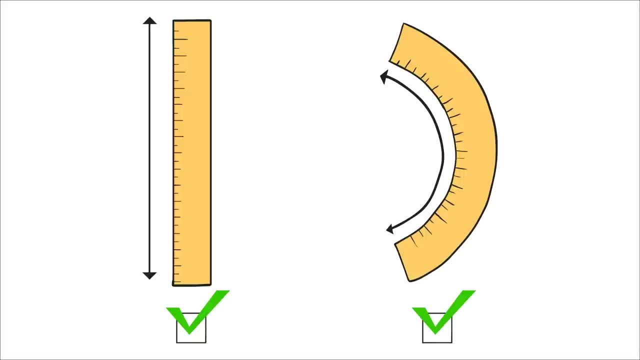 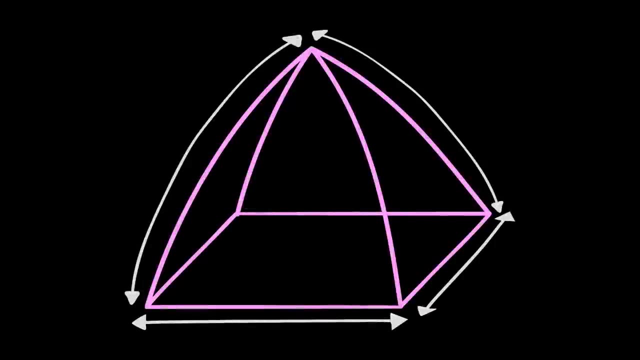 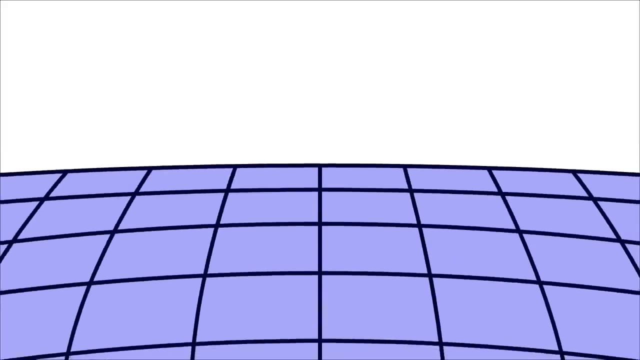 And yet these images are as true, as logically well-constructed as anything we see in Euclid. And when this geometry got to three dimensions, it unveiled a horrific revelation. Why would these parallel lines curve away from each other? Well, because the planes they were on were not flat. 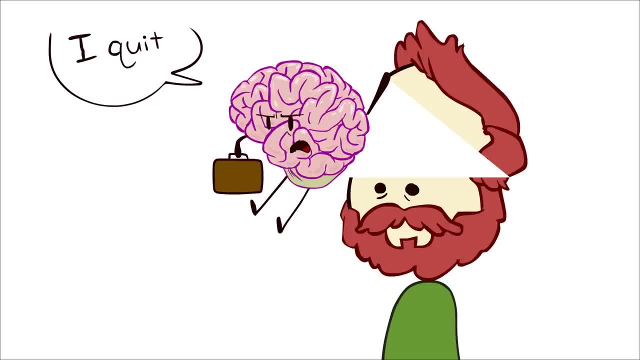 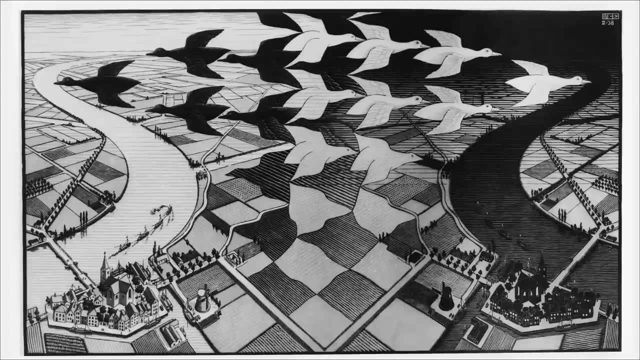 The very space they existed in was curved. For many, this was mind-breaking. What, No, What? 130 years later, this would serve as the foundation for parts of MC Escher's art. But this new geometry was good for more than just art. 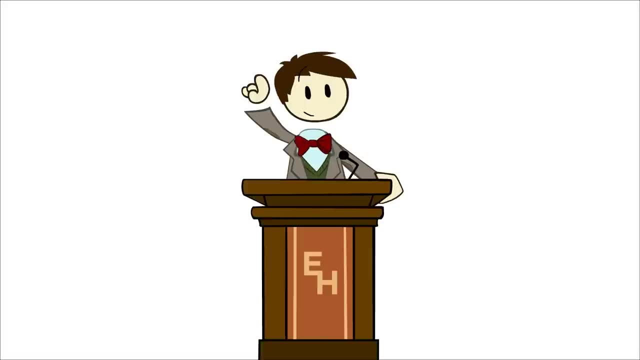 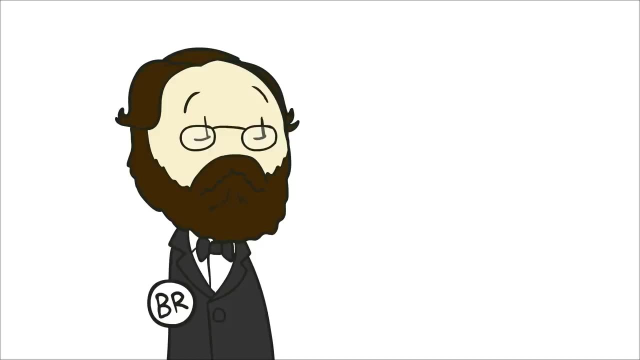 This new understanding opened up a whole world of formulas to create and theorems to develop. It expanded what people thought of as possible, And one of those people was a man named Bernard Riemann. Riemann saw that there were other possibilities for non-Euclidean geometry. 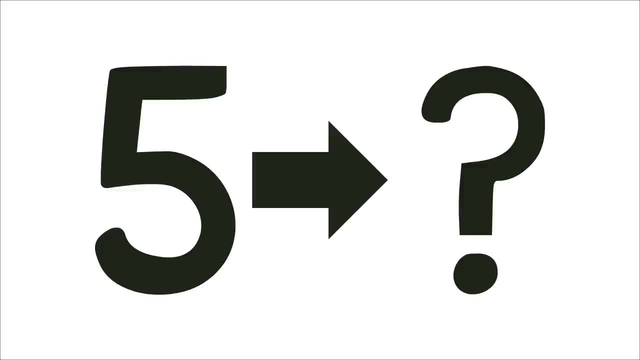 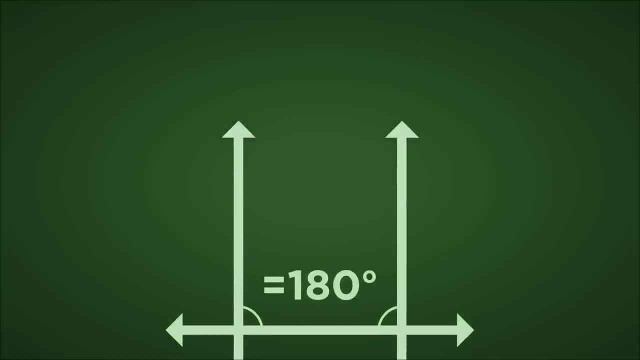 The simplest was the second case. we stated for possible alternatives to postulate 5, the case in which lines whose interior angles add up to exactly 180 degrees don't stay equidistant but actually get closer to one another. How is this possible, you might ask. 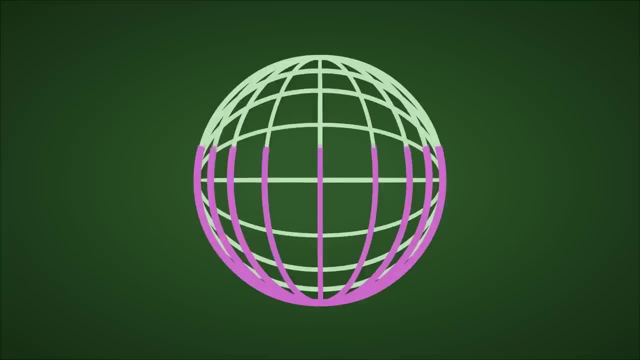 Well here, Imagine a globe. Think about the lines of longitude on a globe. You can lay a line across them that should make them parallel, by our Euclidean postulate, And yet they all intersect. Any line of longitude you choose will cross all other lines of longitude at the poles. 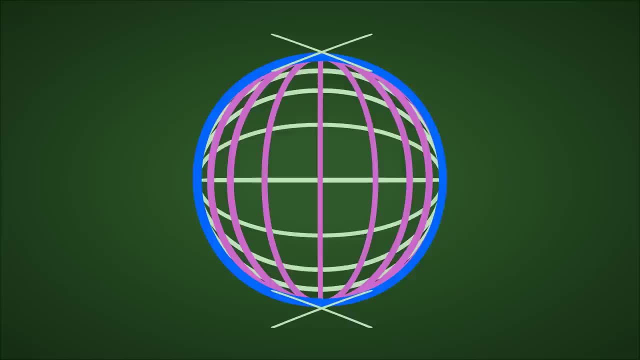 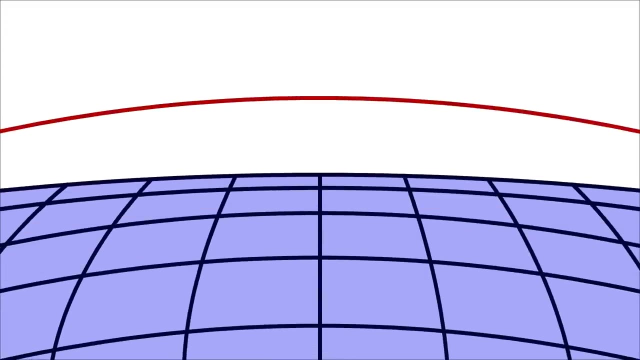 In fact, in this context, the very idea of lines starts to break down. If your flat plane is actually a globe, you simply can't draw a straight line. As soon as you start to extend that line at all, it has to be curved. 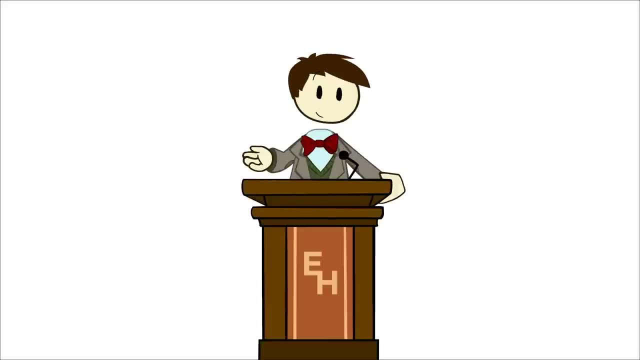 Moreover, some of the things that we had come to understand about lines by this point in history, like the idea that between any two points you can draw one and only one unique line, completely break down. I mean, if you take the poles on a globe as our two points. 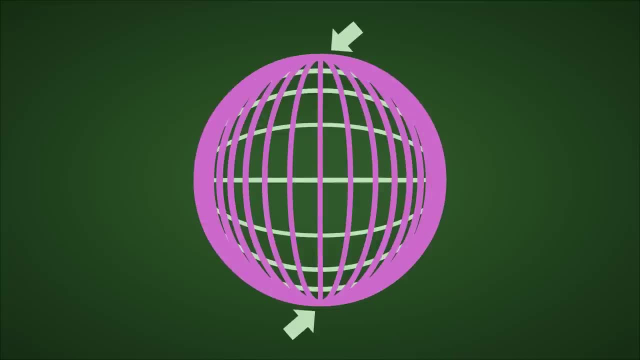 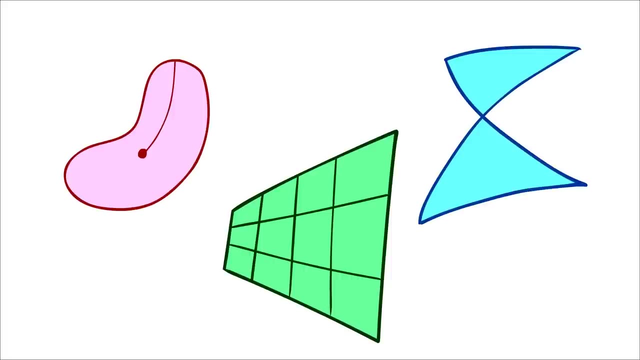 there are infinitely many lines that I can extend from one to the other, And this, like with Bolyai and Lobachevsky's earlier hyperbolic geometry, does strange and unnatural-seeming things to our shapes When you add up the angles in a triangle. 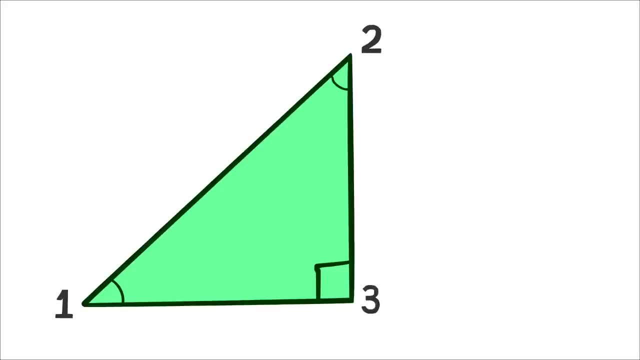 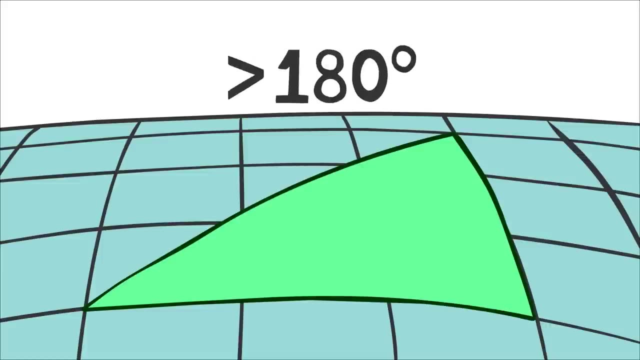 how many do you get? Well, on a normal Euclidean plane you get the sum of two right angles. But here, on our hyperbolic surface, here our triangle's angles add up to more than two right angles and our squares 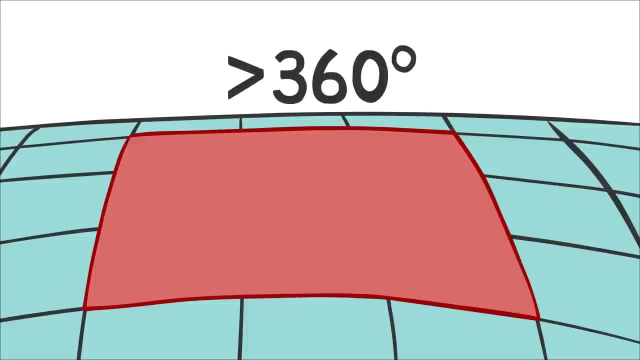 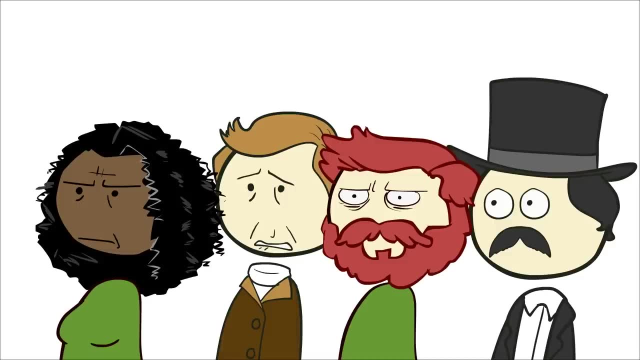 as much as such a concept is even still possible. all have angles that add up to more than four right angles. Now, this may all seem batty. In fact, to most people at the time, and even to most people today, it feels uncomfortable. 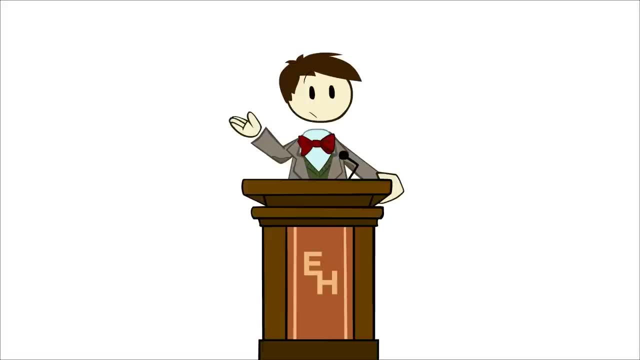 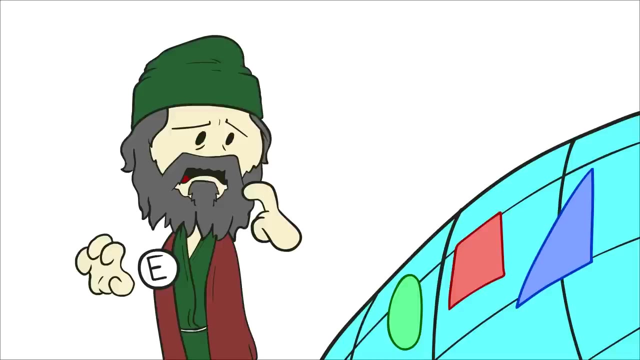 wrong or just hard to grasp. After a lifetime of training your brain to think of objects like columns or spheres in Euclidean space, it can be almost impossibly difficult to start thinking of space as spherical or curved or bent, and the implications that has on geometry. 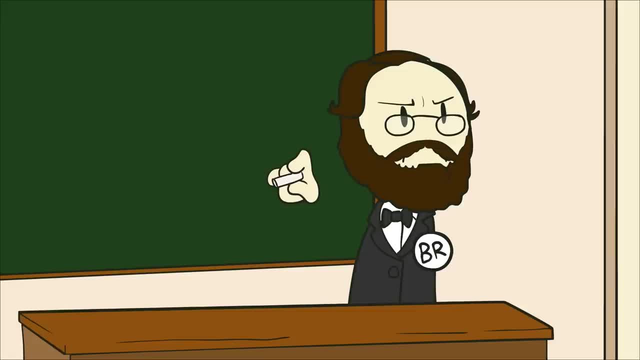 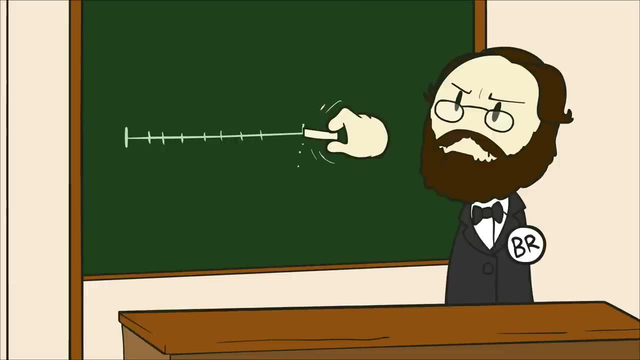 But Riemann did it. In fact, he did it in an extraordinary way. Standing in a lecture hall in front of a small crowd, at barely 26 years of age, Riemann began to unfold an idea. he had an idea that would change everything. 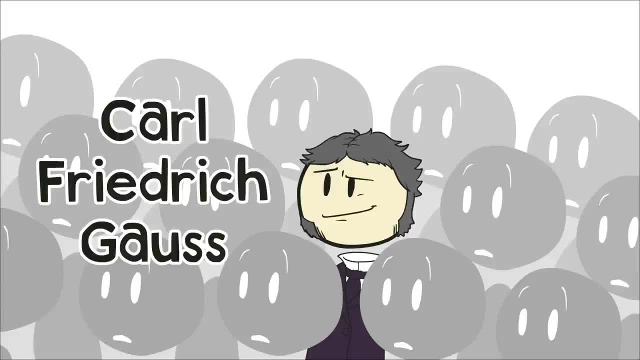 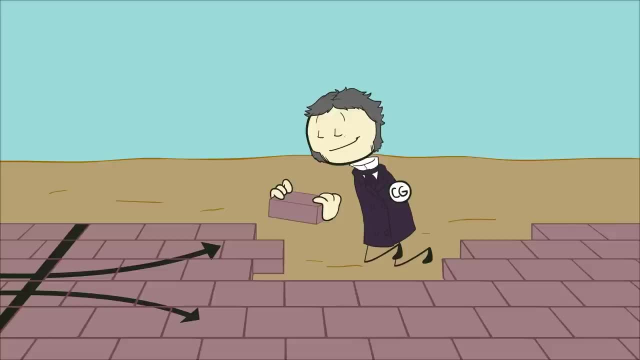 In this small crowd sat his old teacher Gauss, one of the foremost minds in mathematics, the person who really laid the foundation for much of the work in non-Euclidean geometry to come, As Riemann began to chalk out his idea on the blackboard. 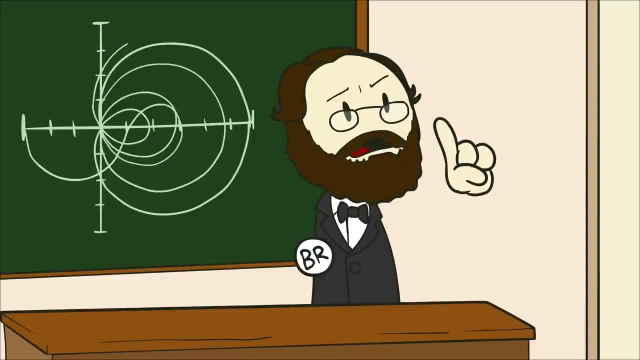 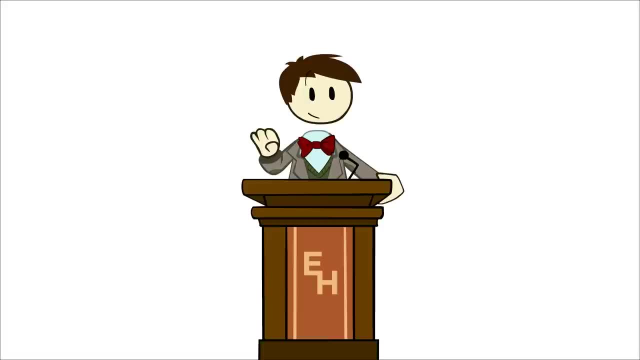 Gauss began to nod with pride. He had known what this lecture would be about, but seeing the details, he knew that even his work had been outdone. Instead of just proposing hyperbolic geometry or the geometry of spherical space, Riemann proposed that there were infinitely many possible non-Euclidean geometries. 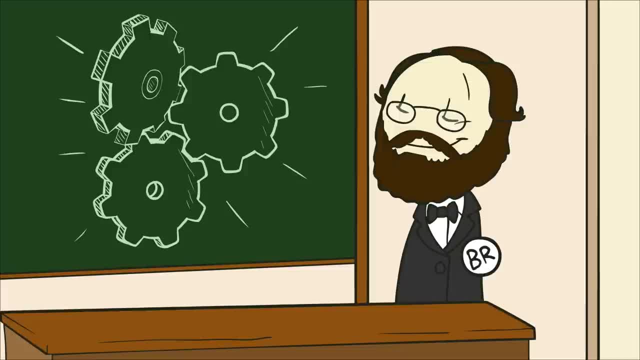 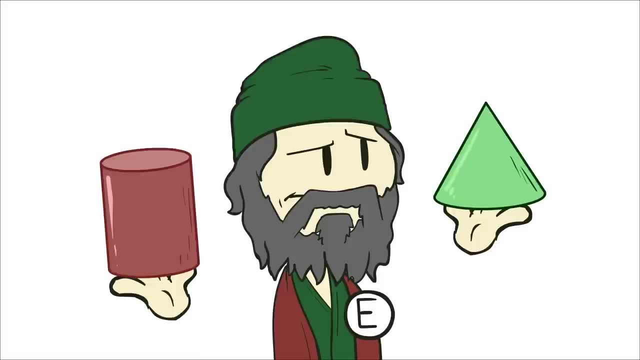 And there, on that chalkboard, he began to lay out what would become a system to unite them all. We wouldn't have to explicate a whole new geometry every time we wanted to look at a new type of curved space. Instead, Riemann suggested that there were mathematical ways of looking at them all. 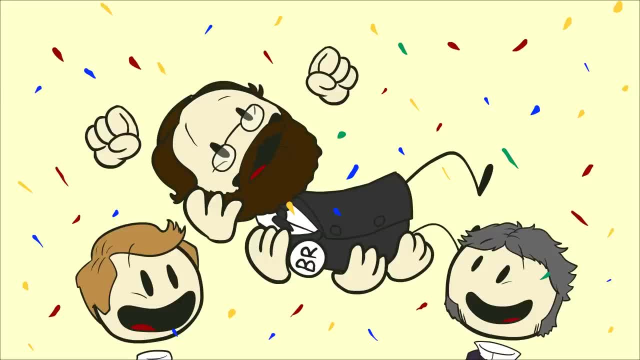 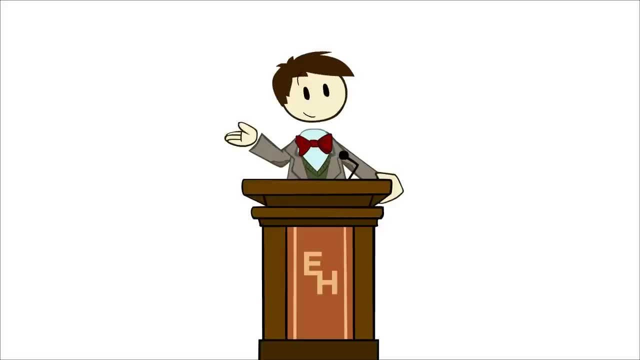 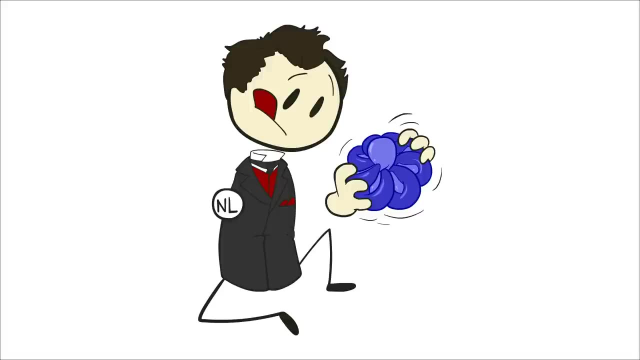 no matter how weird or how complicated. And this is incredibly important because by having a unified theory of non-Euclidean space, regardless of dimensions or shape, it means that non-Euclidean geometry might no longer be just a mathematical curiosity, It might no longer be an abstract mathematical plaything. 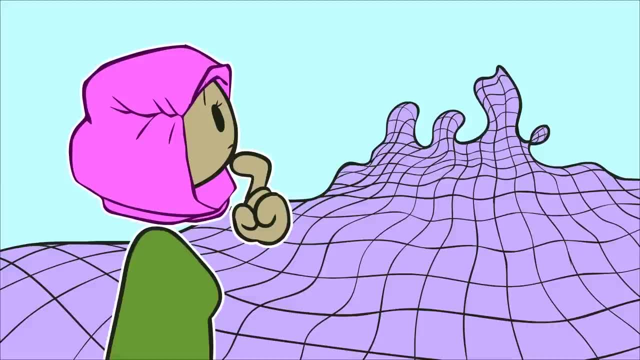 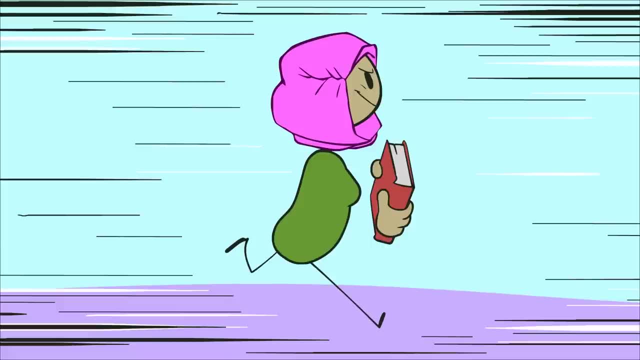 for the brightest minds to toy with. Instead, it means that if we were ever to find an area of reality where our Euclidean laws break down, we now have a system for investigating it mathematically, whatever it might be. And guess what? 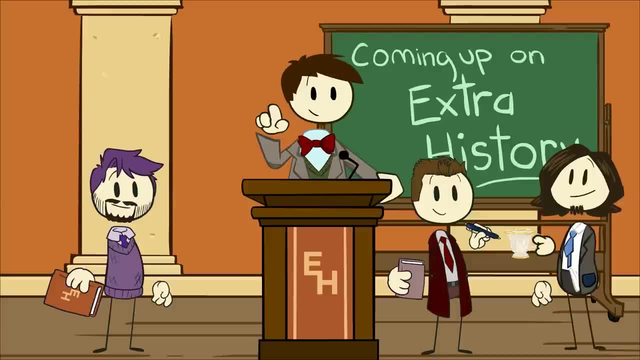 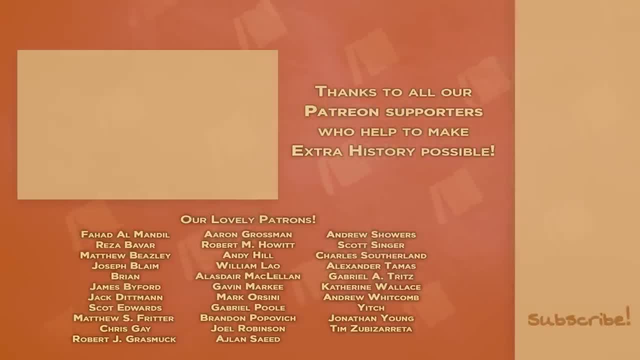 Next episode we are going to find the place where exactly that happens. Thanks for watching.